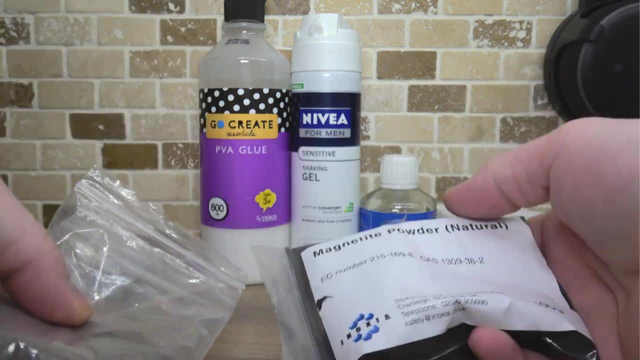 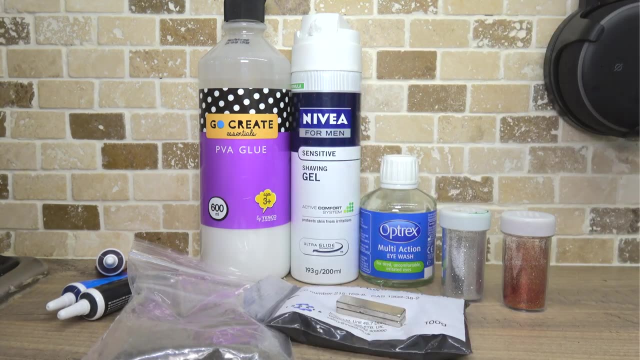 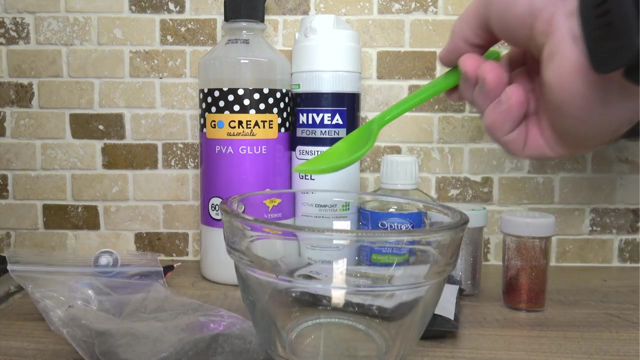 Here. we've got some magnetite powder and some iron filings. You only need one of these and we've got a magnet to play with the slime once we made it. We put some links in the description below where you can get the magnetic items from And, of course, something to mix it in. It won't stain your bowl. 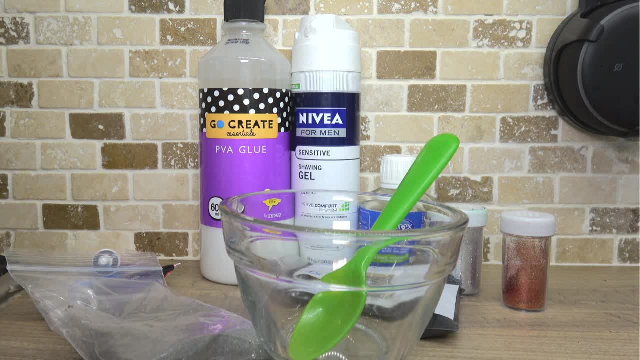 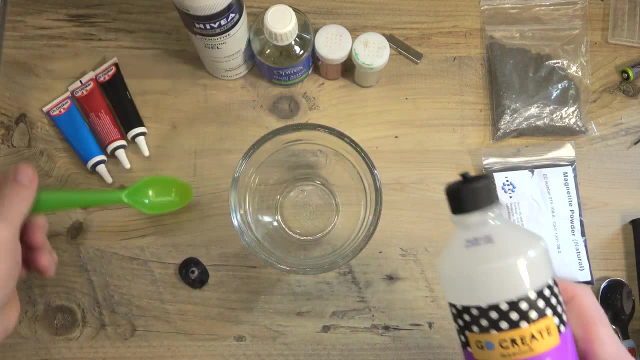 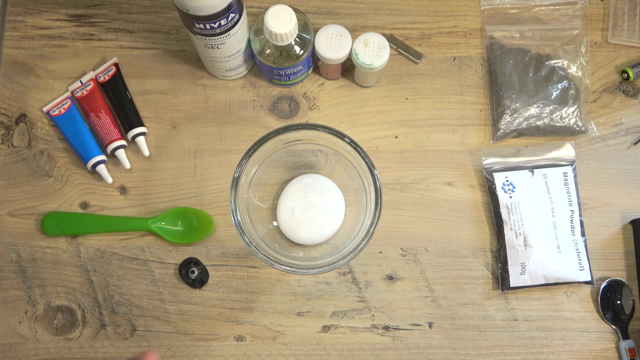 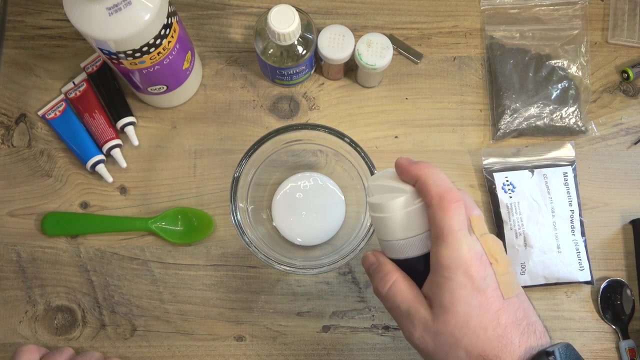 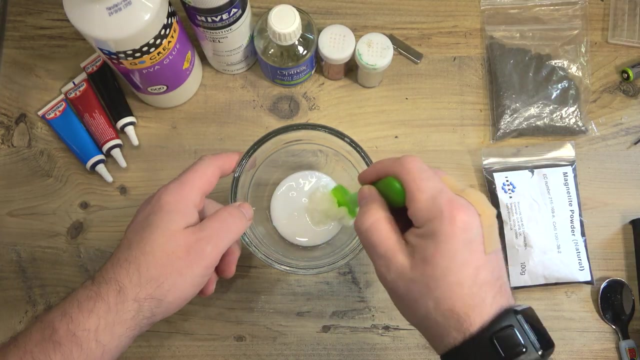 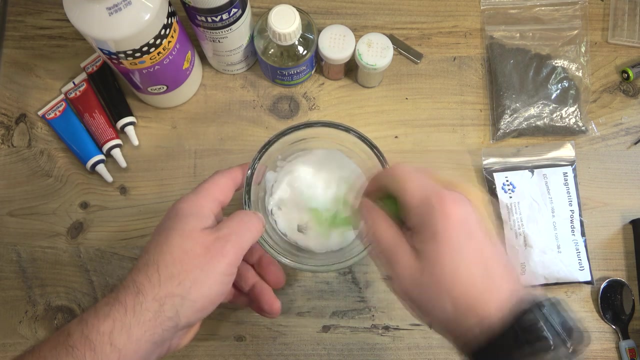 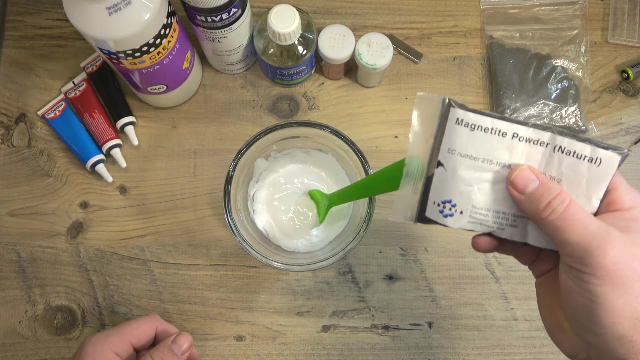 but it's probably best not to tell your wife if you're using a good one. Okay, down to business. Put a good squirt of PVA in the bowl And then a big squirt of shaving foam. Mix it together. As I'll be using the magnetite powder for this slime, it'll make the slime look pretty much black. 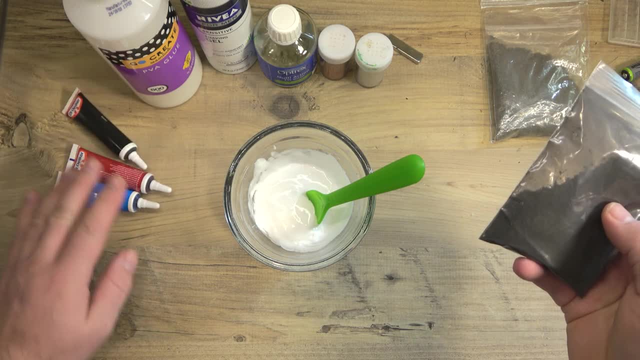 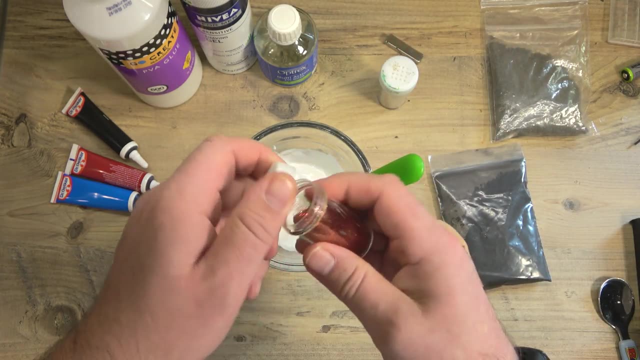 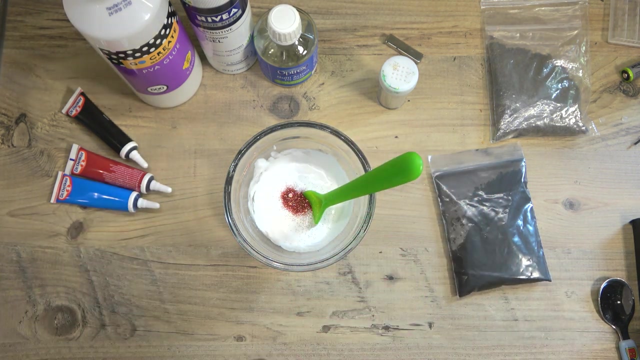 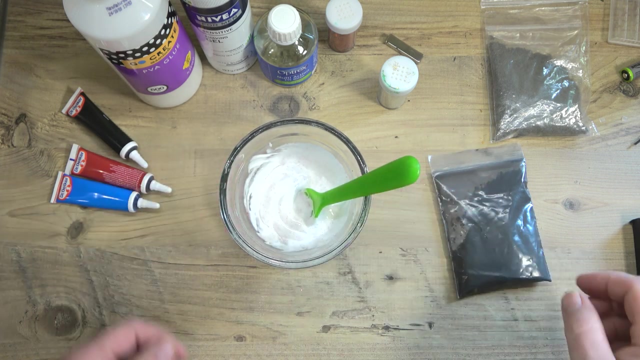 So there's no point in adding any food colouring. However, a bit of glitter will make it look great. I'm going to add some red glitter and give it a good mix up. Once the glitter is mixed in, it's time to add some magnetite. 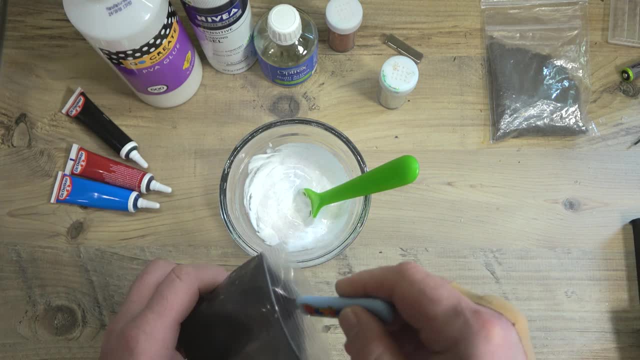 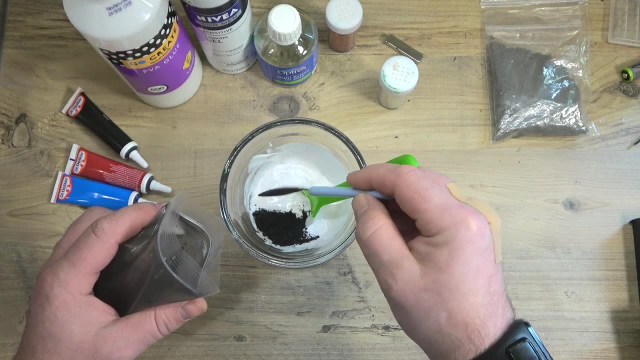 I'm going to add about a teaspoon: The more you add, the more attracted to a magnet it will be, So it's worth experimenting. This would be the same for the iron filings. Give that a good mix up. And now for the magic ingredients. 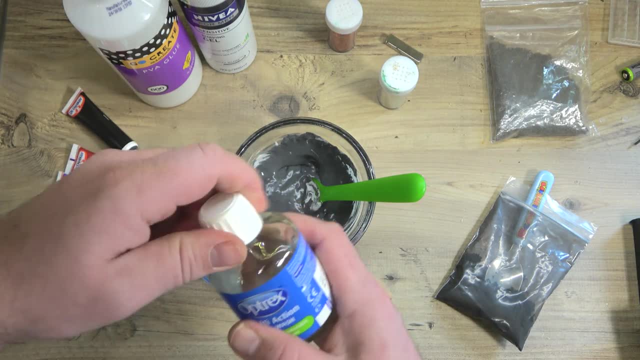 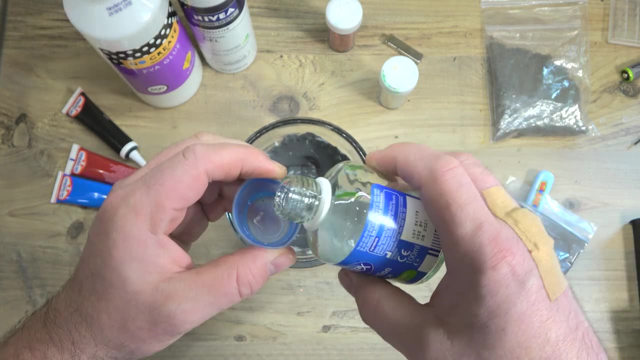 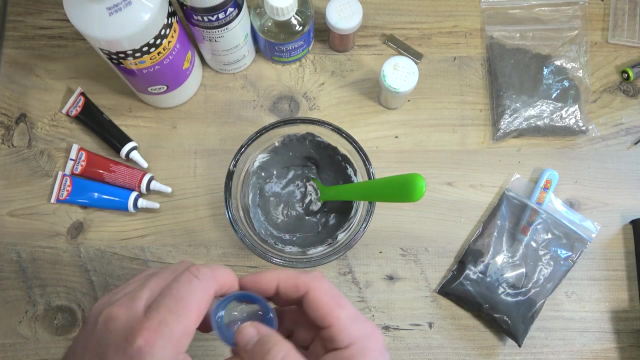 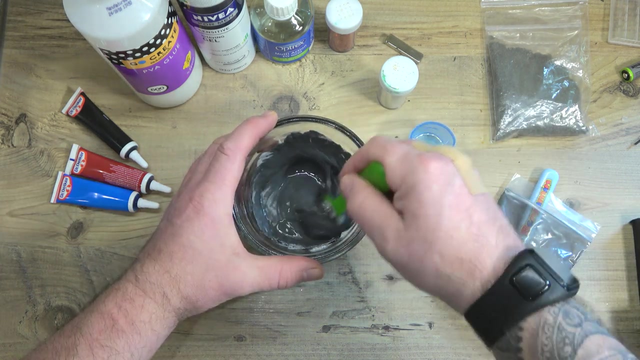 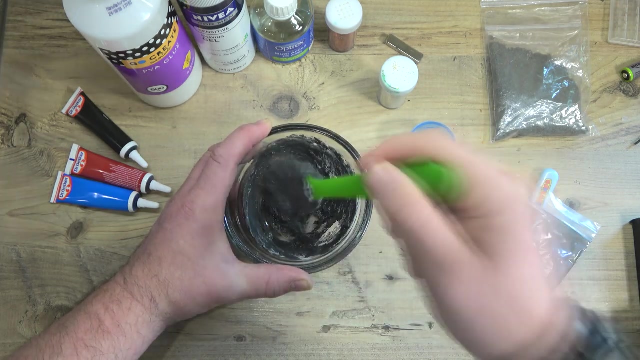 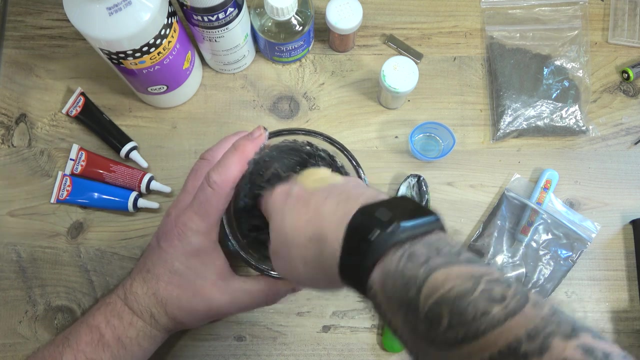 Ok, now we're ready for the magic ingredients. You only need to add a few drops to the mix. Here I'm probably using about half a teaspoon. Give it another good mix and you'll very quickly feel it get firm and sticky. Once it's kind of stuck together as one lump, take it out of the bowl and work it between.